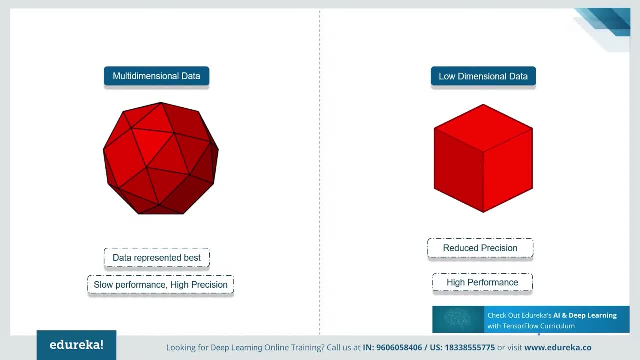 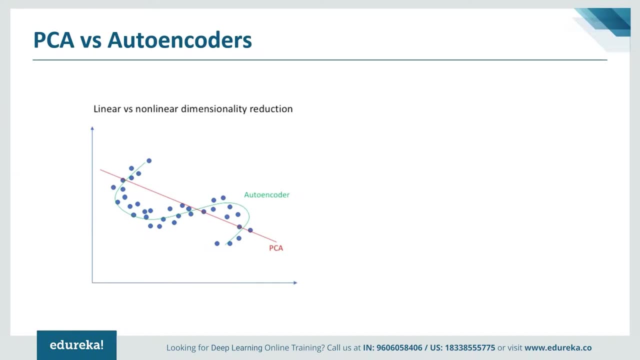 Typically for the purpose of dimensionality reduction. now, for that we already have principal component analysis. Then why do we need auto encoders? So an auto encoder can learn nonlinear transformations, unlike PCA with a nonlinear activation function and multiple layers. now it doesn't have to learn dense layers. 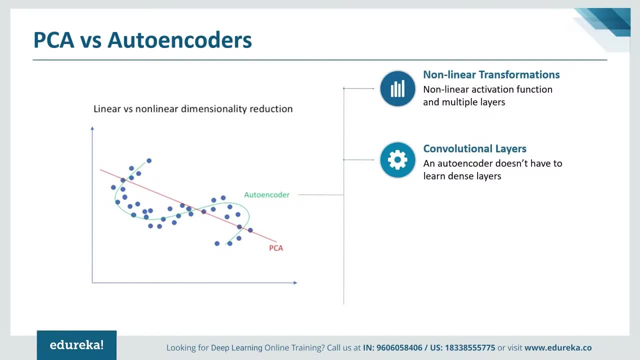 So it can use convolutional layers to learn to, which could be better for video image and series data. Now it may be more efficient in terms of model parameters to learn several layers with an auto encoder rather than learn one huge transformation with PCA, and auto encoder also gives a representation. 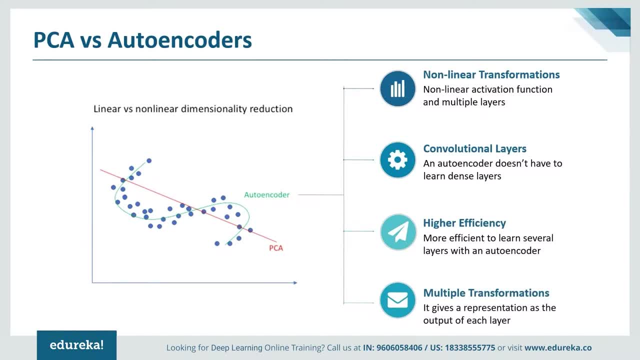 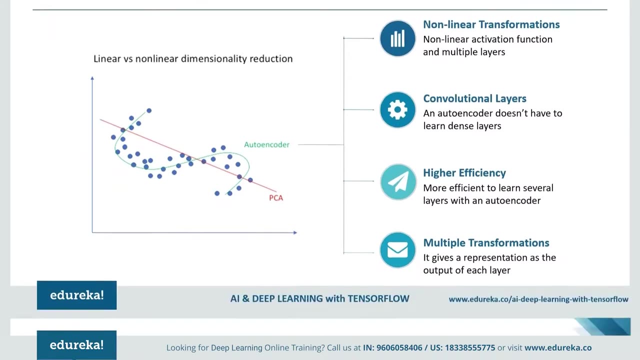 as the output of each layer and having multiple representations of different dimensions is always useful. So an auto encoder could let you make use of pre-trained layers from another model to apply transfer learning to prime the encoder or the decoder. despite the fact that the practical applications 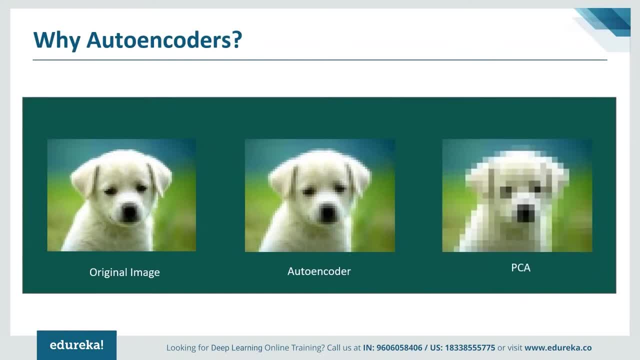 of auto encoders were pretty rare sometime back today, data denoising and dimensionality reduction for data visualization are considered as two main interesting practical applications of auto encoders. now, with appropriate dimensionality and sparsity constraints, auto encoders can learn data projections that are more interesting than PCA or other basic techniques. 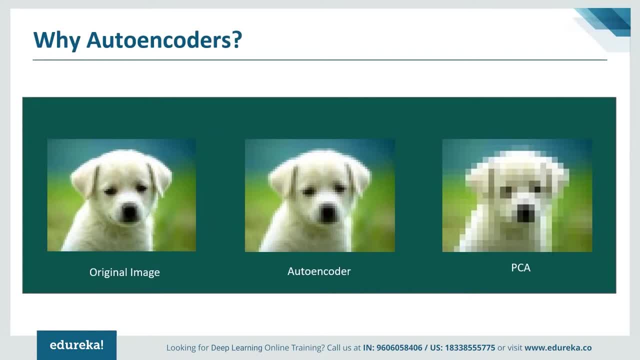 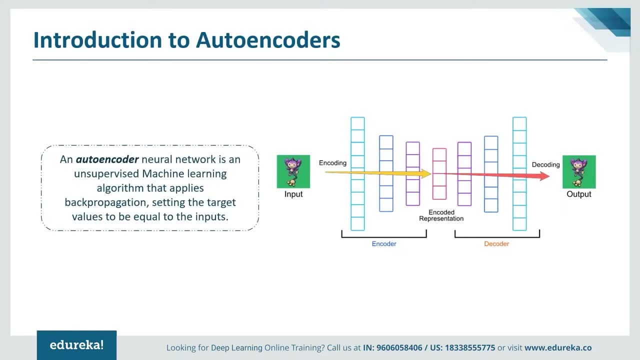 It also provides a more accurate output when compared to PCA. now, auto encoders are simple learning networks that aim to transform inputs into outputs with the minimum possible error. This means that we want the output to be as close to input as possible and auto encoder neural network. 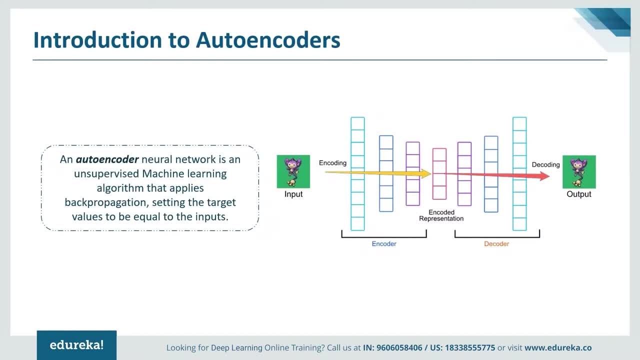 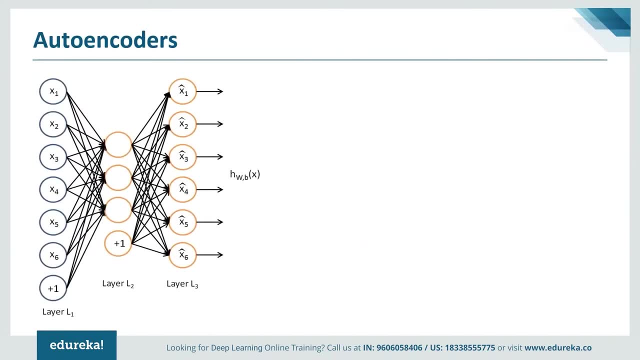 is basically an unsupervised machine learning algorithm that applies back propagation, setting the target values to be equal to the inputs. So let's have a look at some of the key features about auto encoders. So it is an unsupervised machine learning algorithm. 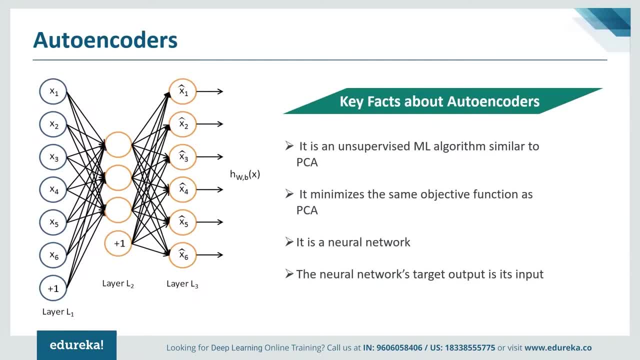 that is similar to PCA but minimizes the same objective function, and auto encoder is a neural network whose target output is its input. auto encoders, Although, is quite similar to PCA, but they are more flexible when compared to the other. auto encoders can represent both linear and nonlinear transformation in encoding. 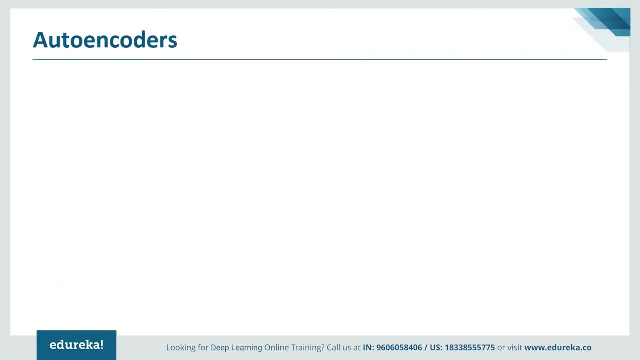 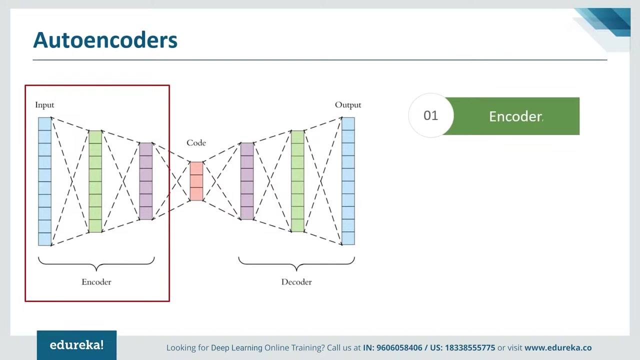 but PCA can only perform linear transformation. So now let's have a look at the components of auto encoder. So there are basically three main layers. The first one is the encoder, then code and decoder. the first component, that is the encoder, is the part of the network that compresses the input. 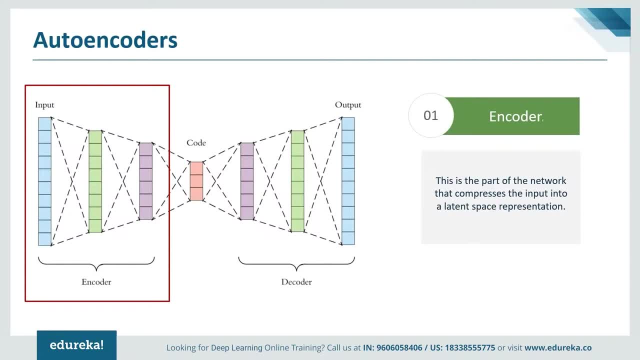 into a latent space representation. the encoder layer encodes the input image as a compressed representation in a reduced dimension. Now the compressed image typically looks garbled, nothing like the original image. the next component represents the latent space. Now code is the part of the network that represents. 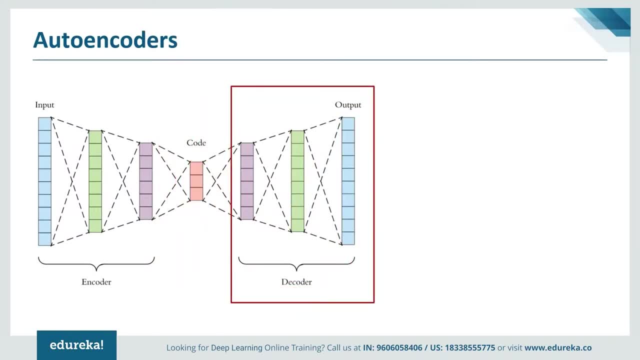 the compressed input fed to the decoder. The third component is a decoder. Now this layer basically decodes the encoded image back to the original dimension. The decoded image is a lossy reconstruction of the original image. Now it reconstruct the input from the latent space representation. 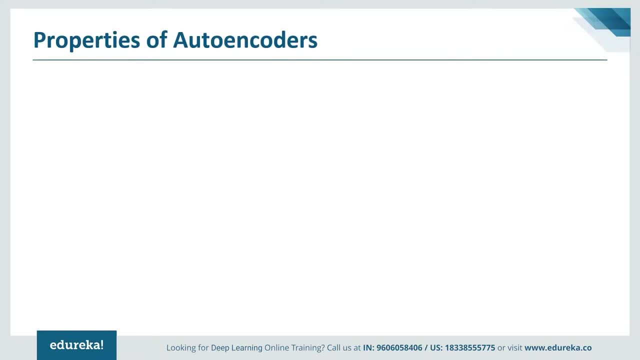 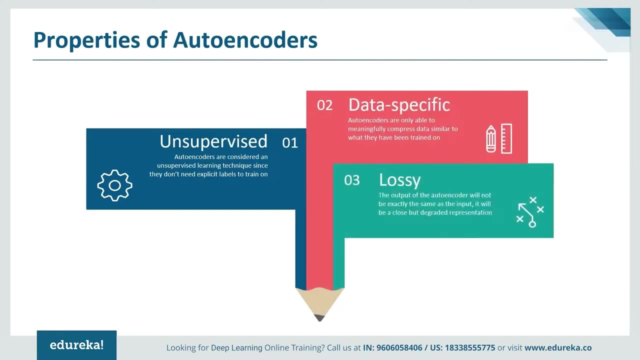 So now let's talk about some of the properties of auto encoders. They are only able to compress data similar to what they have been trained on. an auto encoder which has been trained on human faces would not be performing well with images of modern buildings. 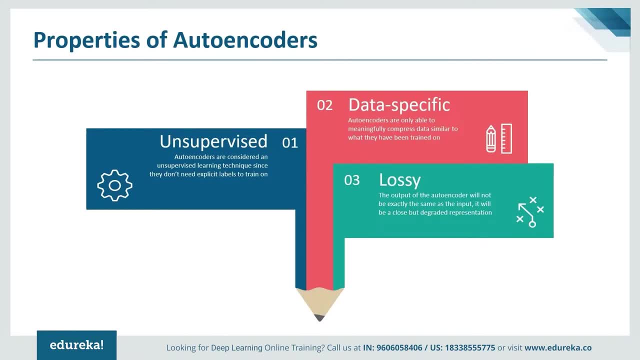 This improvises the difference between the auto encoders and mp3 kind of compression algorithms, which only hold assumptions about sound in general but not about specific types of sounds. auto encoders are lossy, which means that the decompressed outputs will be degraded compared to the original inputs. just 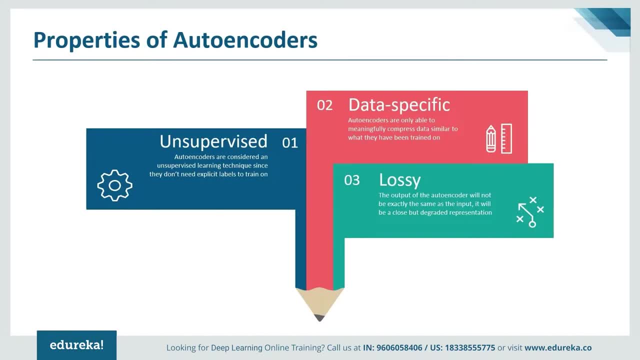 like what you see in JPEG or mp3.. Now, if you have appropriate training data, it is easy to train specialized instances of the algorithm that will perform well on a specific type of input. Now it doesn't require any new engineering. Additionally, in almost all contexts, 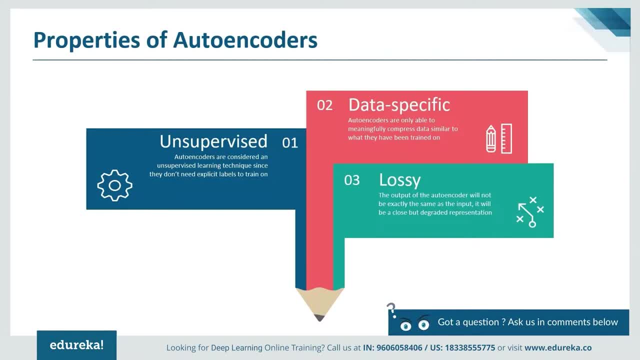 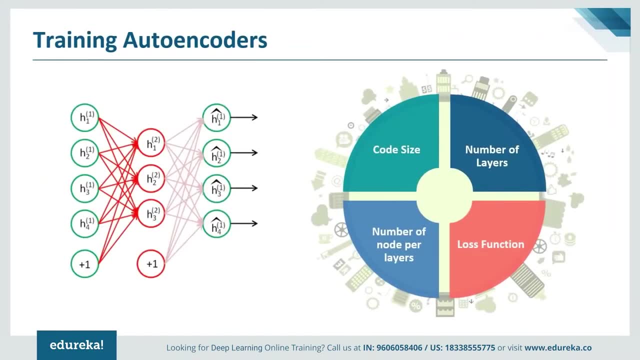 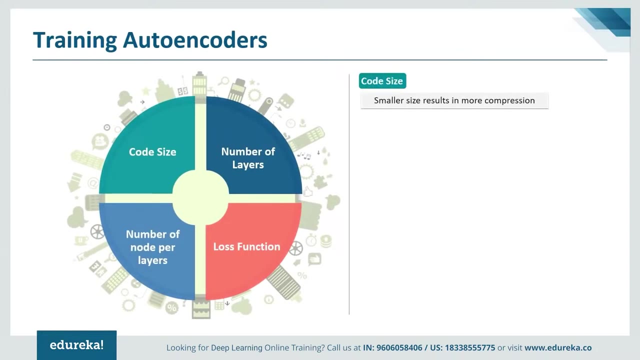 where the term auto encoder is used. the compression and decompression functions are implemented with neural networks. So now let's have a look at the training of an auto encoder. Now there are four hyper parameters that we need to set before training them. The first one is the code size. the code size represents 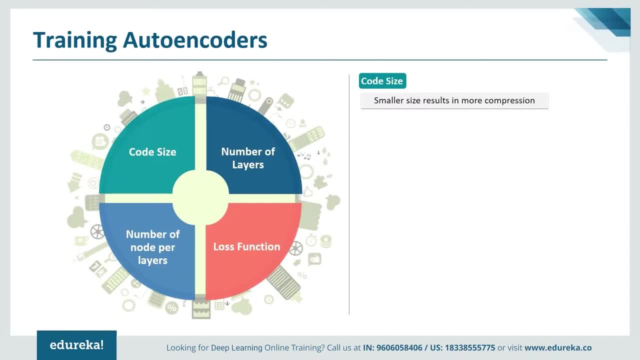 the number of notes in the middle layer. smaller size results in more compression. The second parameter is the number of layers. Now the auto encoder can be as deep as we want it to be. We can have two or more layers in both the encoder and decoder, without considering the input and the output. 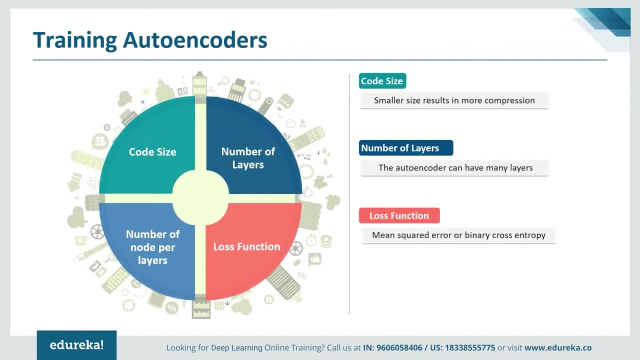 Next is the loss function. So we either use mean squared error or binary cross entropy. Now, if the input values are in the range 0 to 1, then we typically use cross entropy. Otherwise we use the mean squared error. next is the number of notes per layer. 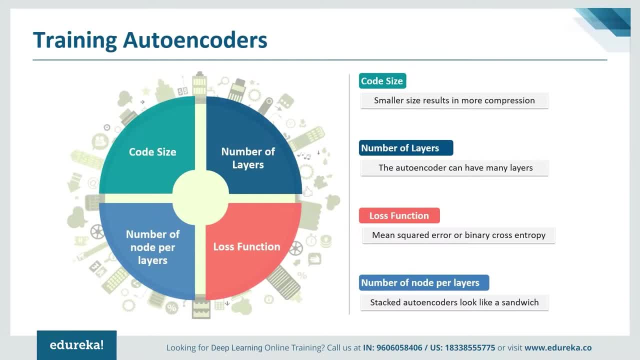 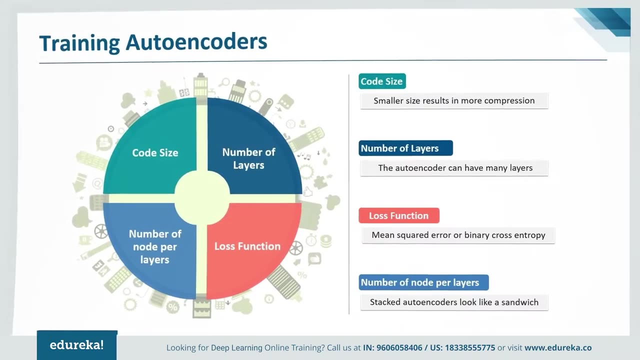 So the number of nodes per layer decreases with each subsequent layer of the encoder and increases back in the decoder. Also, the decoder is symmetric to the encoder in terms of layer structure, but this is not necessary and we have total control over these parameters. Now let's have a look at the architecture. 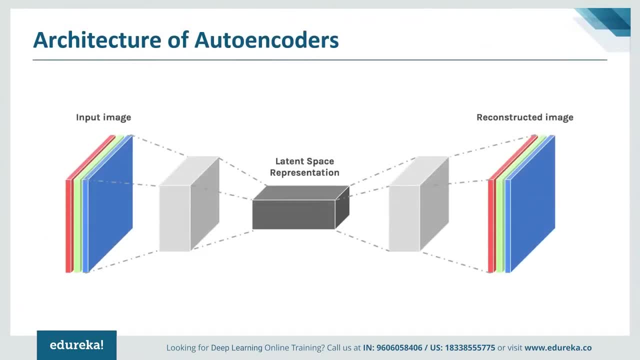 of an auto encoder and have a deeper insight about the hidden layers. So in an auto encoder we add a couple of layers in between the input and output and the sizes of these layers are smaller than the input layer. Let's say the input vector has a dimensionality of n. 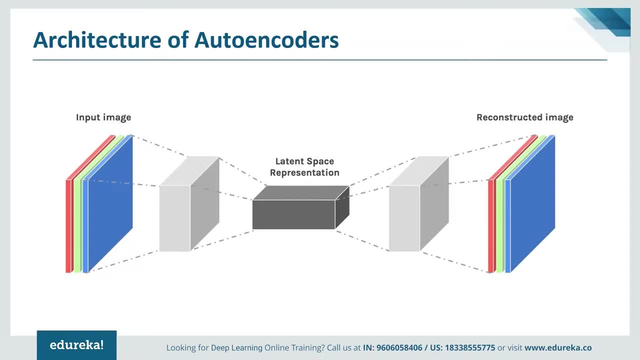 which means that the output will also have a dimensionality of n. now we make the input go through a layer of size P, where the value of P is less than n, and we ask it to reconstruct the input. Now the auto encoder receives unlabeled input. 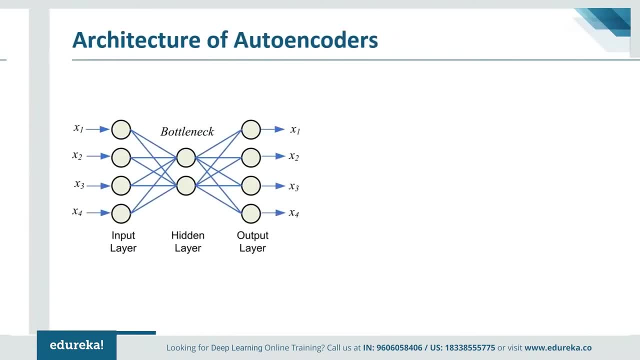 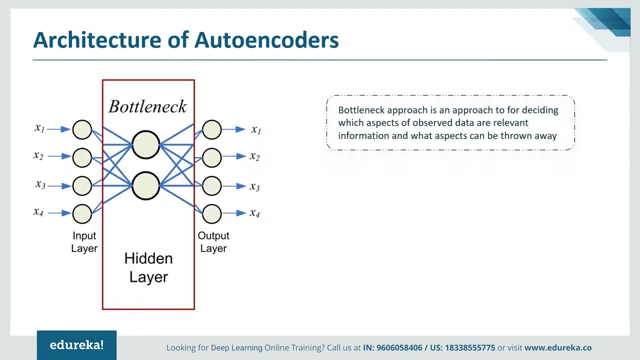 which is then encoded to reconstruct the input. one important part of the auto encoders is the bottleneck. Now, the bottleneck approach is a beautifully elegant approach to a representation learning specifically for deciding which aspects of observed data are relevant information and what aspects can be thrown away. 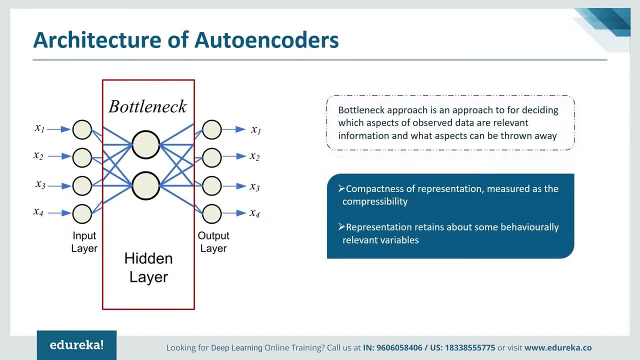 It does this by balancing two criteria, that is, the compactness of representation, measured as the compressibility number- number of bits needed to store the representation- and the second one information the representation retains about some behaviorally relevant variables. Now it assumes we know what the behaviorally relevant variables are. 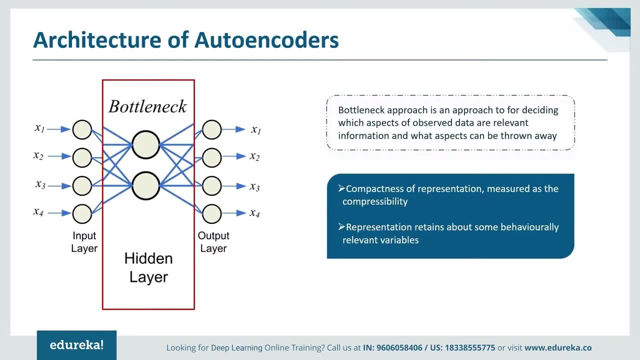 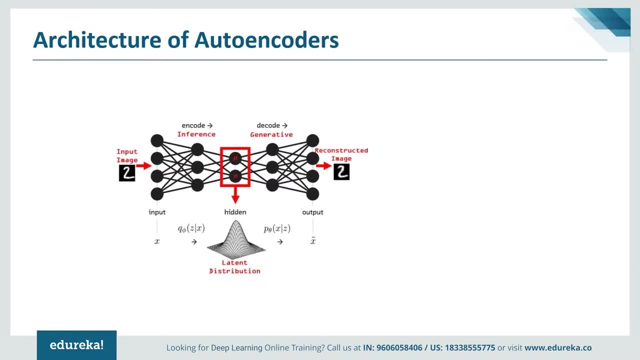 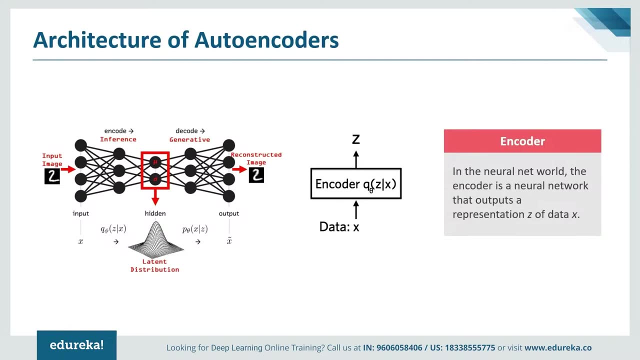 and how they are related, to observe data- or at least we have to have data- to learn or approximate the joint distribution between observed and relevant variables. Now let's have a detailed description about the encoder. The encoder is a neural network. Its input is a data point X, its output. 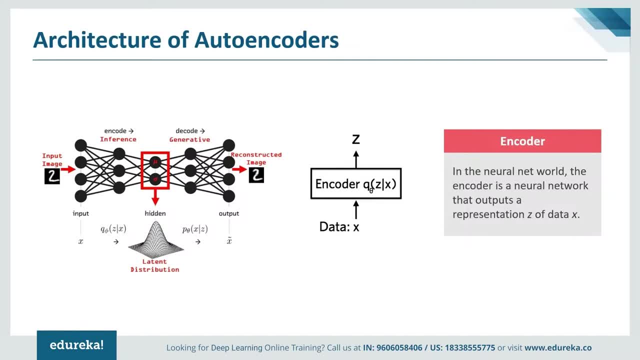 is a hidden representation Z, and it has weights and biases, Theta. now to be concrete, Let's say X is a 28 by 28 pixel photo of a handwritten number. The encoder encodes the data, which is 784 dimensional, into a latent representation space, Z. 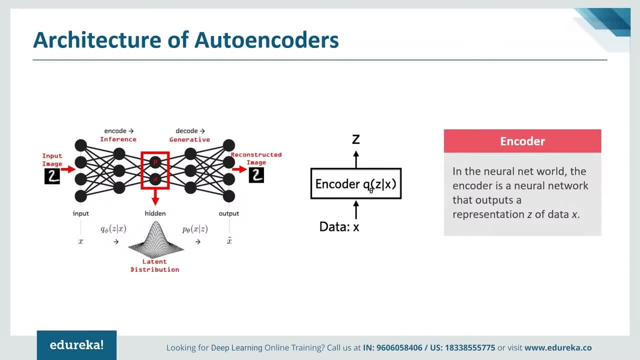 which is much less than 784 dimensions. Now this is typically referred to as a bottleneck, because the encoder must learn an efficient compression of the data into this lower dimensional space. next is the decoder. The decoder is another neural net. its input is the representation Z. it outputs the parameters. 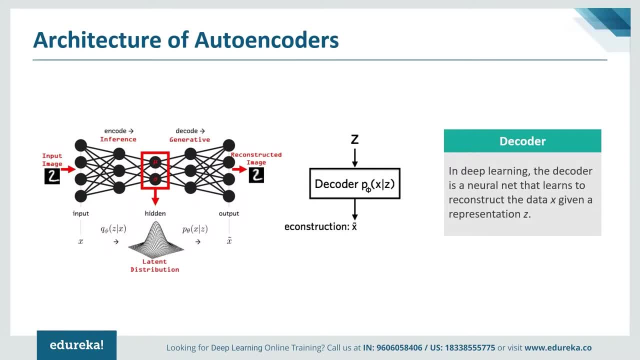 to the probability distribution of the data and has weights and biases as Phi. running with the handwritten digit example, Let's say the photos are black and white and represent each pixel as 0 or 1. now the probability distribution of a single pixel can be then represented using a Bernoulli distribution. 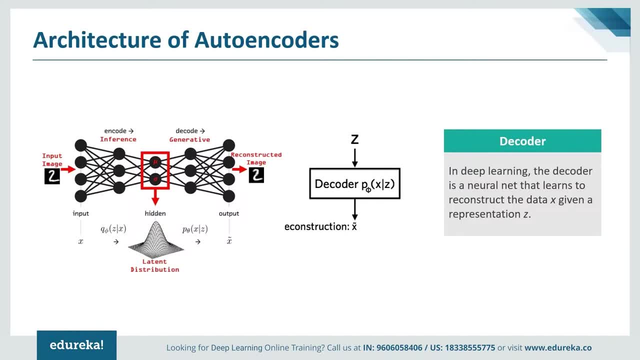 The decoder gets as input the latent representation of a digit Z and outputs 784 Bernoulli parameters, one for each of the 784 pixels in the image. The decoder decodes the real valued numbers in Z into 784 real valued numbers between 0 and 1 information. 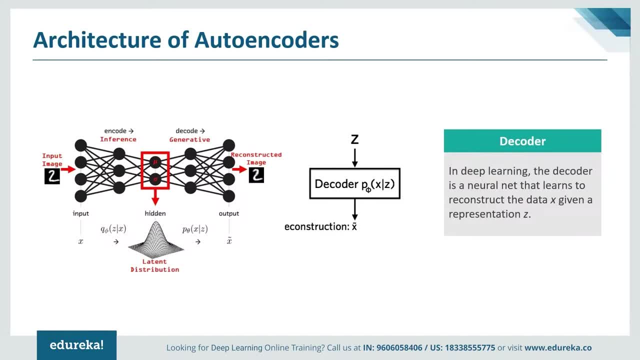 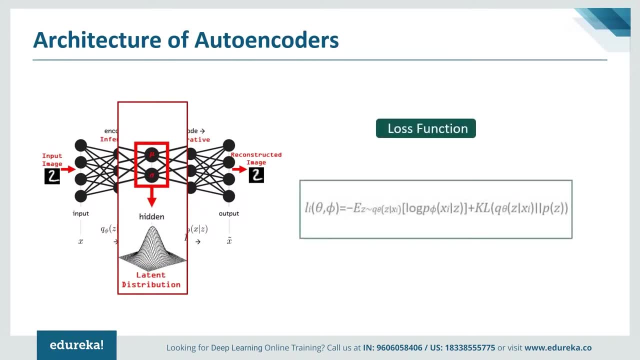 is lost because it goes from a smaller to a larger dimensionality. Now how do we find out how much information is lost? The loss function equation helps us find the value. Now this measure tells us how effectively the decoder has learned to reconstruct an input. image X given. 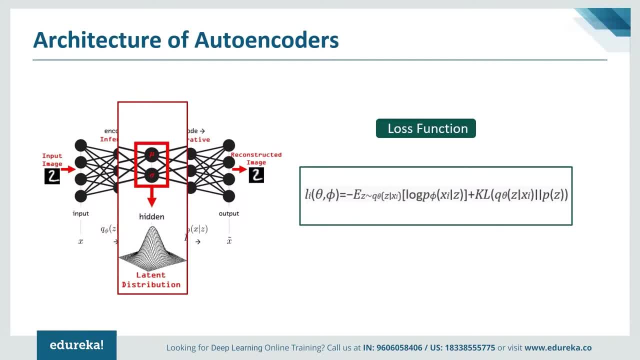 its latent representation Z. the loss function of the variational autoencoder is the negative log likelihood with a regularizer. because there are no global representations that are shared by all data points, We can decompose the loss function into only terms that depend on a single data point. 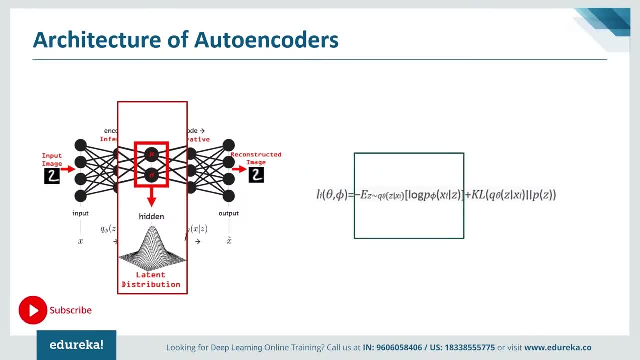 So the loss function. the first term is the reconstruction loss or expected negative log likelihood of the i-th data point. The expectation is taken with respect to the encoders distribution over the representations. This term encourages the decoder to learn to reconstruct the data. Now, if the decoders output does not reconstruct the data, 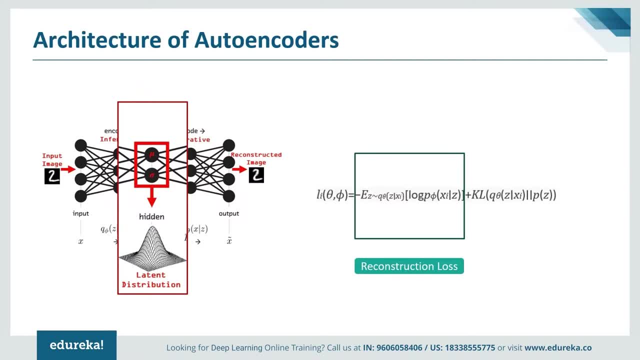 Well, it will incur a large cost in the loss function. The second term is a regularizer that we throw in. this is the callback labeler. Divergence between the encoders: distribution. Now, this Divergence measures how much information is lost when using Q to represent P. it is one measure. 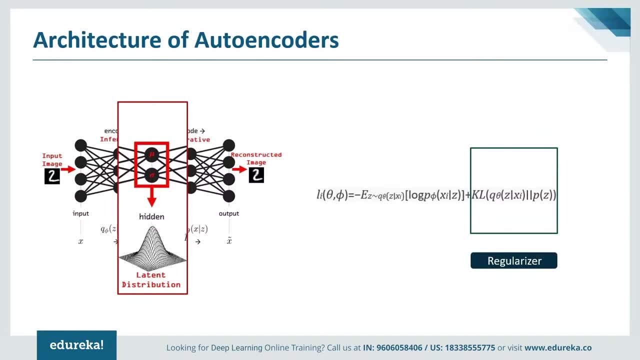 of how close Q is to P. if the encoder outputs representations said that are different than those from a standard normal distribution, It will receive a penalty in the loss. this regularizer term means keep the representation Z of each digit sufficiently diverse. if we didn't include the regularizer, the encoder could learn. 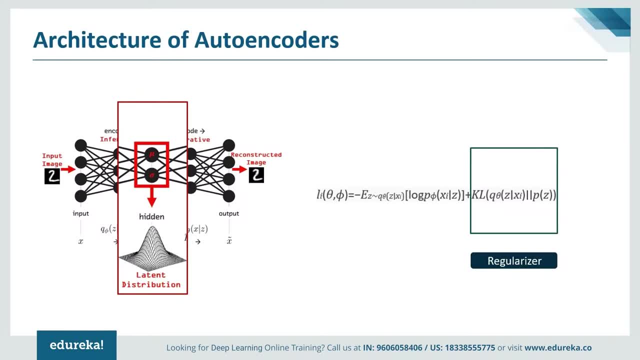 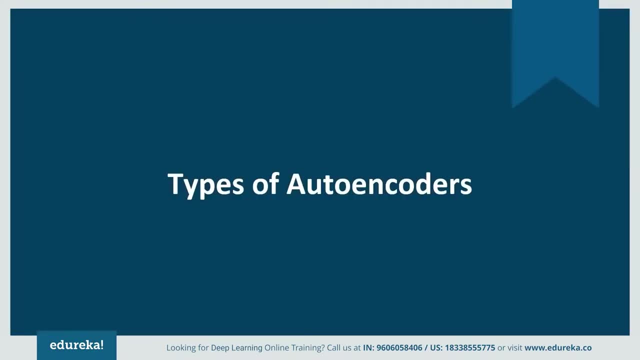 to cheat and give each data point a representation in a different region of Euclidean space. So now let's move on and have a look at the different types of auto encoders. The convolution operator allows filtering and input signal in order to extract some parts. 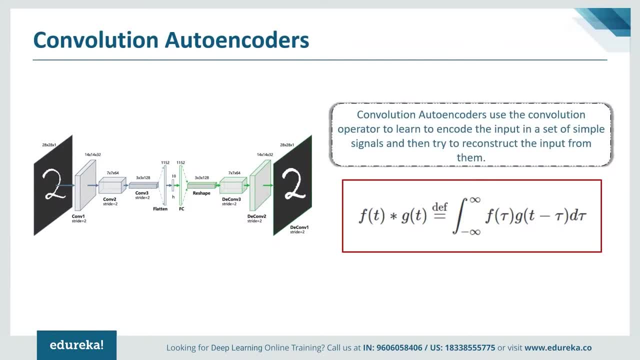 of its content. auto encoders, in their traditional formulation, do not take into account the fact that the signal can be seen as a sum of other signals. convolution: auto encoders use the convolution operator to exploit this observation. Basically, they learn to encode the input in a set. 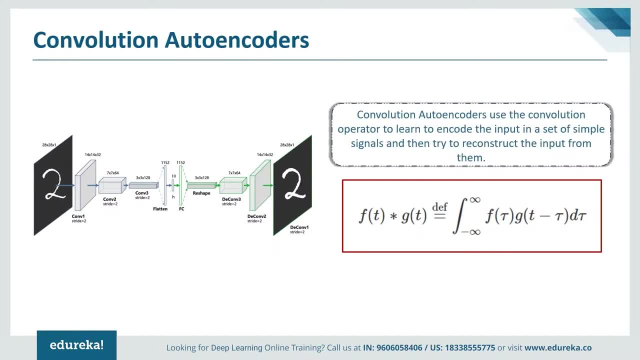 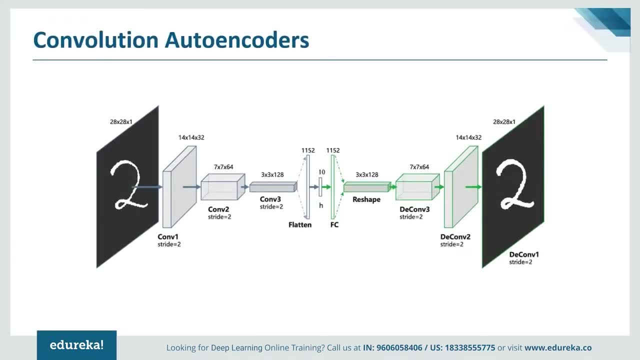 of simple signals and then try to reconstruct the input from them, modify the geometry or the reflectance of the image. Now the encoder consists of three convolutional less. the number of features changes from one, the input data, to 16 for the first convolutional layer, then from 16 to 32. 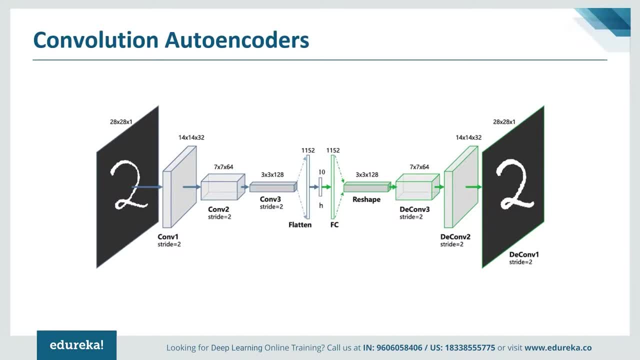 for the second layer, and finally, from 32 to 64 for the final convolutional layer. now, while transacting from one convolutional layer to another, the shape undergoes an image compression. So the decoder consists of 3d convolution layers and instant sequence for each deconvolution operation. 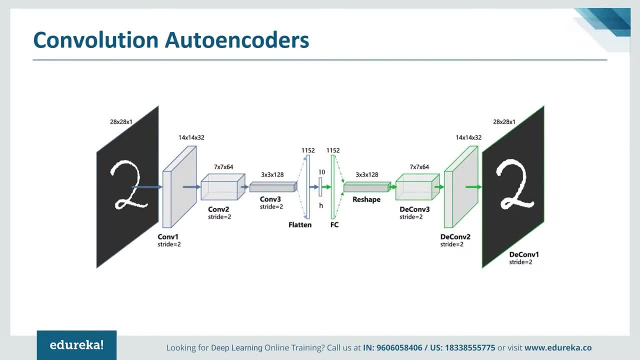 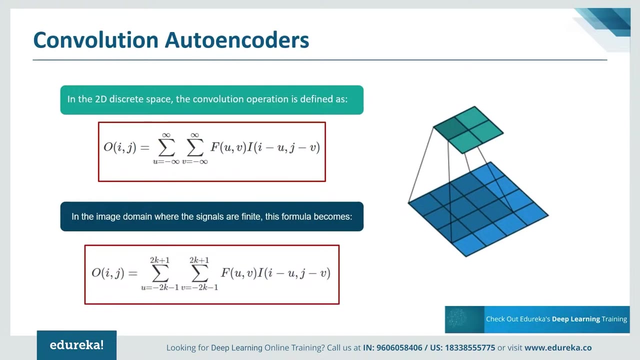 We reduce the number of features. to obtain an image, that must be the same size as the original image. So, in addition to reducing the number of features, deconvolution involves a shape transformation Of the images. a convolution is the general continue case, defined as the integral of the product of two functions. 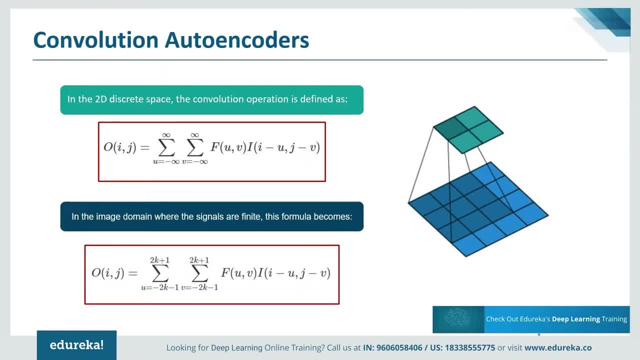 after one is reversed and shifted. as a result, a convolution produces a new function and it is a commutative operation. Now, in the 2d discrete space, the convolution operation is defined as the following equation: and in the image domain, where the signals are finite: 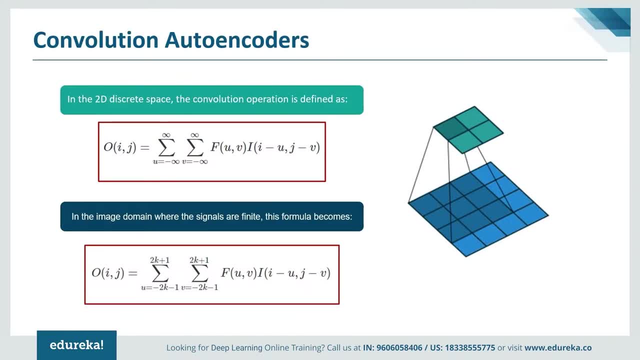 this formula becomes as such: where o of i, j is the output pixel in position i, n, j, and 2 k plus 1 is the side of a square. that is the odd convolutional filter. F is the convolutional filter and I is the input image. 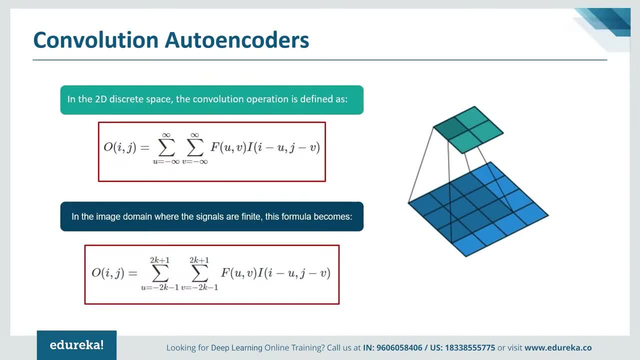 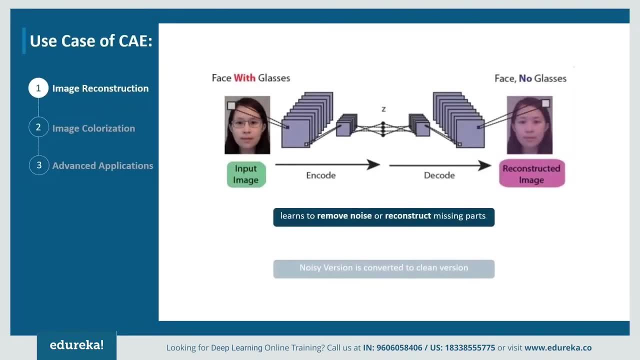 Now this operation is done for every location of the input image that completely overlaps with the convolutional filter. Now let's see the use cases of convolution autoencoders. The first one is image reconstruction. Now the convolution autoencoders learn to remove. 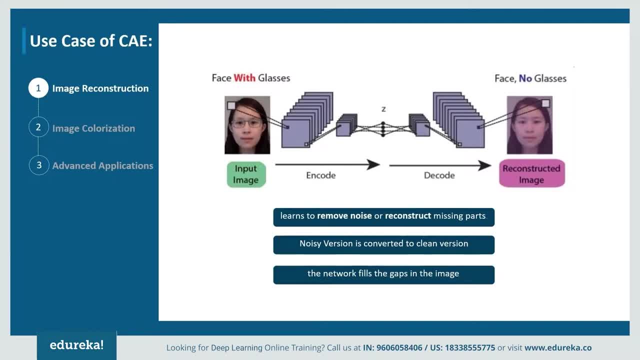 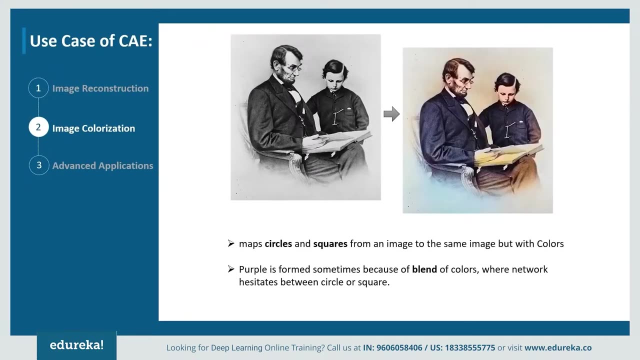 noise from a picture or reconstruct the missing parts. So the input noisy version becomes the clean output version. the network also fills the gap in the image. Next is image colorization. now convolution: autoencoders maps circles and squares from an image to the same image. 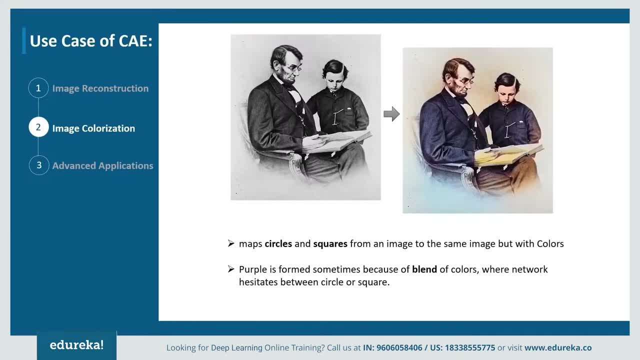 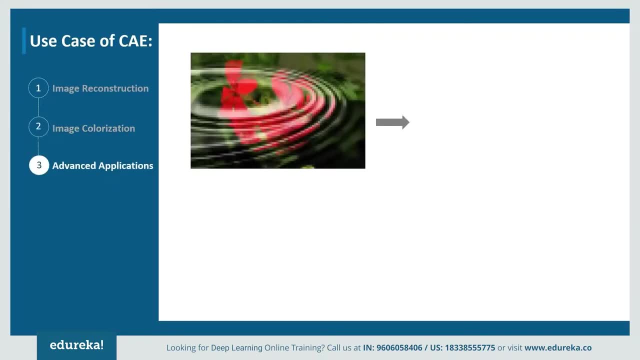 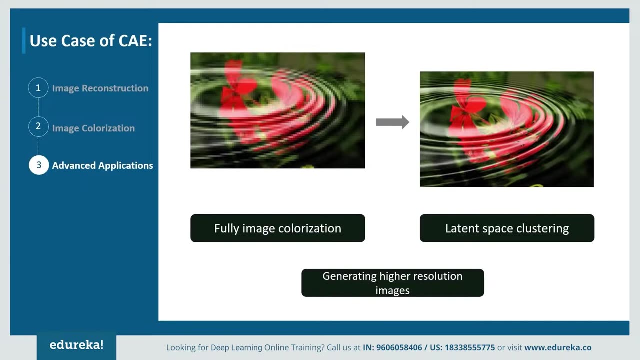 but with red and blue respectively. purple is formed sometimes because of blend of colors where network hesitates between circle or square. next up are some of the advanced applications, such as fully image colorization, latent space clustering and generating high resolution images. moving on to the next type of autoencoders: sparse autoencoders. 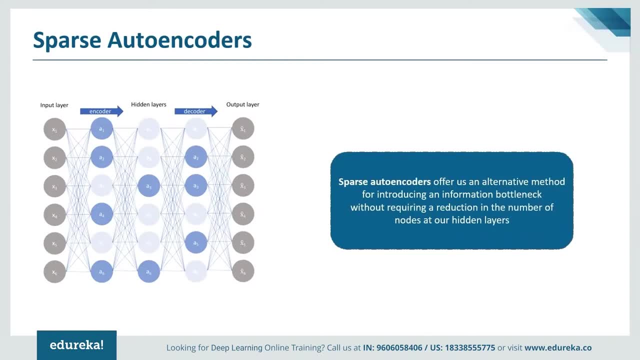 offer us an alternative method for introducing an information bottleneck without requiring a reduction in the number of notes at our hidden layers. Rather, we will construct our loss functions such that we penalize activations within a layer. So for any given observation, we will encourage our network to learn an encoding. 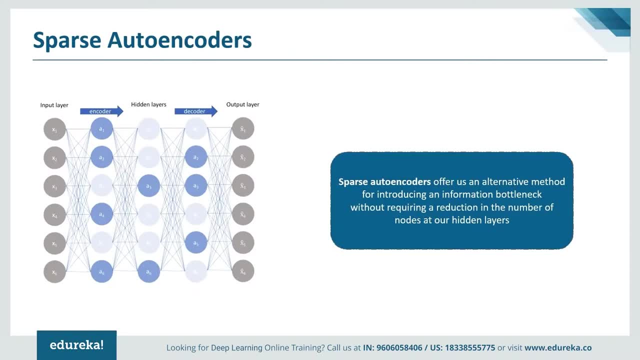 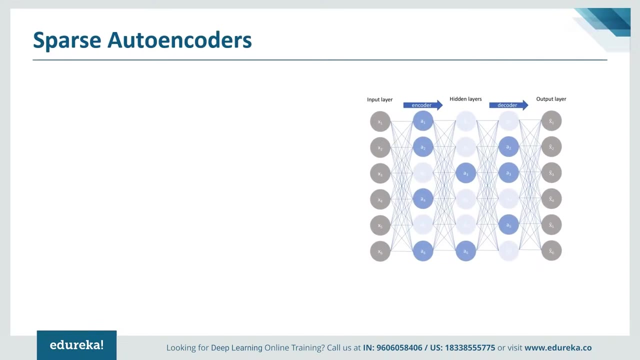 and decoding, which only relies on activating a small number of neurons. Now, this is a different approach towards regularization, as we normally regularize the weights of a network, not the activations. now there are two main ways by which we can impose this parsity constraint. both involve measuring. 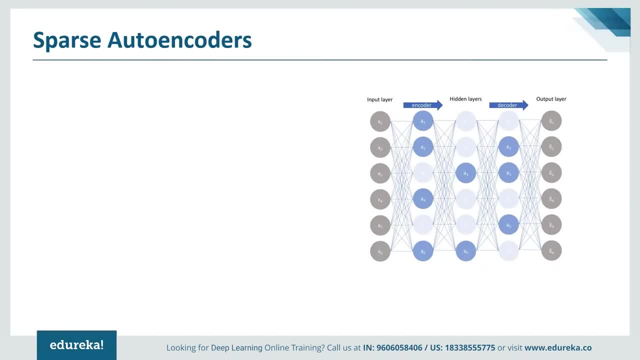 the hidden layer activations for each training batch and adding some term to the loss function in order to penalize excessive activations. The first one is the l1 regularization. Now we can add a term to our loss function that penalizes the absolute value of the vector. 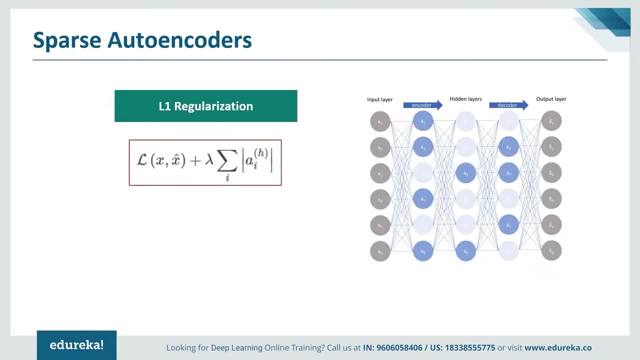 of activations a in layer H for observation. I now scaled by a tuning parameter Lambda. The next one is the KL divergence. in essence, KL divergence is a measure of the difference between two probability distributions. We can define a sparsity parameter row which denotes the average activation of a neuron. 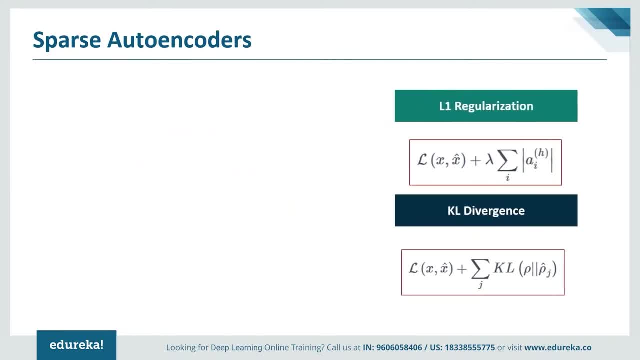 over a collection of samples. This expectation can be calculated in the following equation: Now the KL divergence between two Bernoulli distributions can be written as such: Now this loss term is visualized below: for an ideal distribution of Rho equals to 0.2. corresponding: 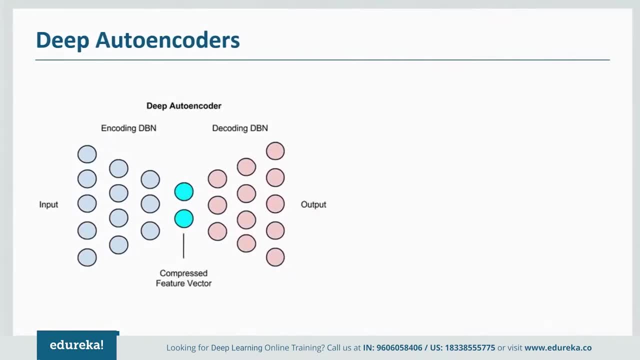 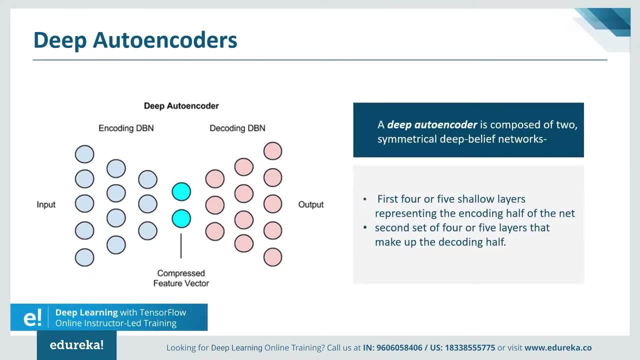 with the minimum penalty at this point. The next one is the deep Auto encoders. Now, the extension of the simple Auto encoder is basically the deep Auto encoders Now. the only difference to its simpler counterpart is number of hidden layers. The additional hidden layers enable the Auto encoder 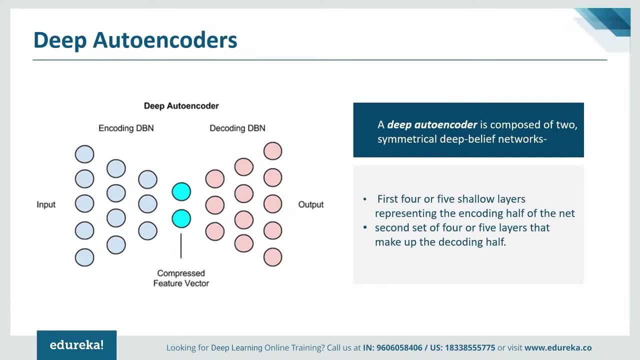 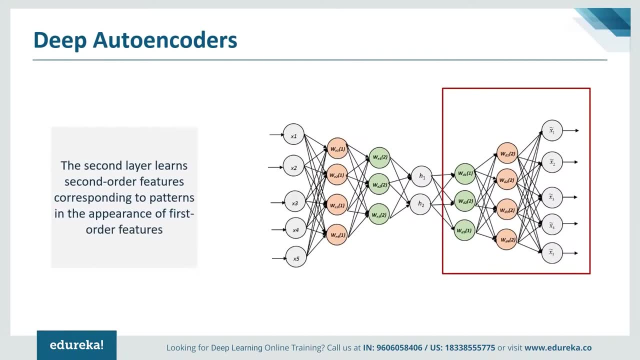 to learn mathematically more complex underlying patterns in the data. The first layer of the deep Auto encoder may learn first-order features in the raw input. The second layer may learn second-order features corresponding to patterns in the appearance of first-order features. deeper layers: 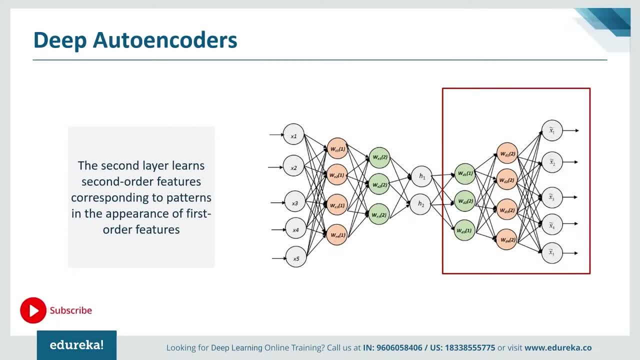 of the deep Auto encoder tend to learn even higher order features. To put everything together, We need additional layers to be able to handle more complex data, such as the data we use in collaborative filtering. So let's have a look at some of the use cases. 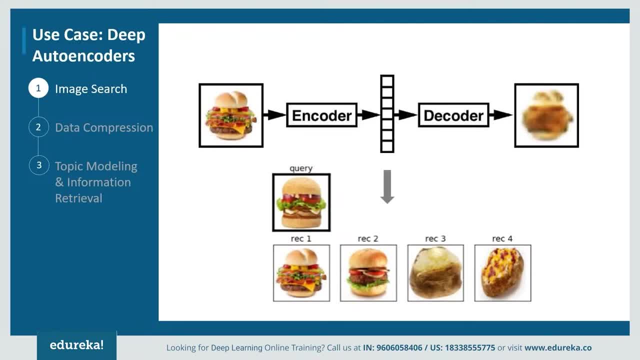 of deep Auto encoders. The first one is image search. deep Auto encoders are capable of compressing images into 30 number vectors. image search therefore becomes a matter of uploading an image, which the search engine will then compress to 30 numbers and compare that vector to all the others in its index vectors. 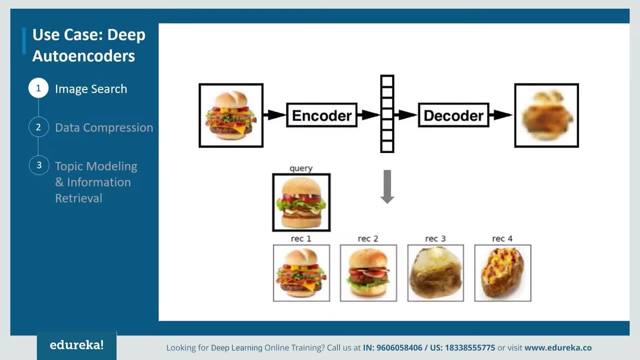 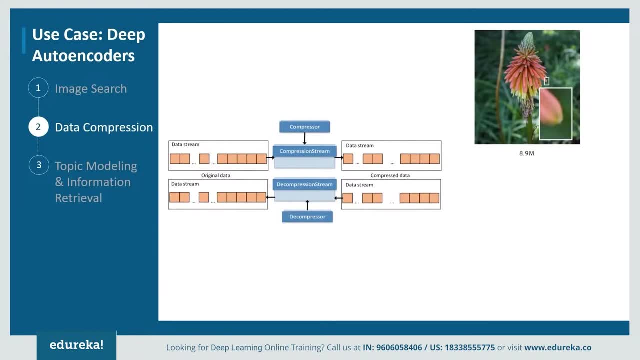 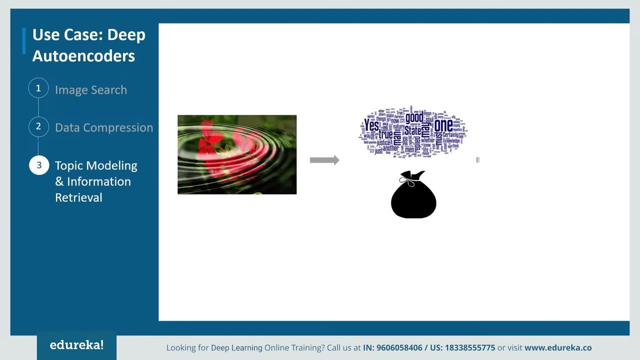 containing similar numbers will be returned for the search query and translated into their matching image. A more general case of image compression is data compression, and deep Auto encoders are useful for semantic hashing. Next up is the topic modeling and information retrieval. So deep Auto encoders are useful in topic modeling. 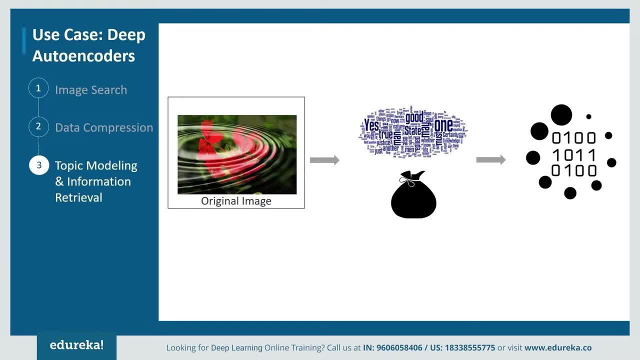 or statistically modeling abstract topics that are distributed across a collection of documents. in brief, Each document in a collection is converted to a bag of words and those word counts are scaled to decimals between 0 and 1, which may be thought of as the probability of a word occurring in the document. 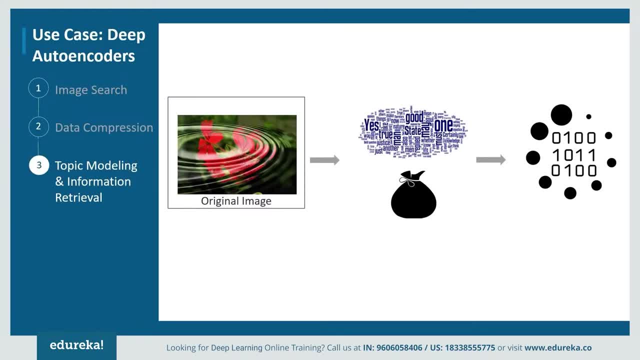 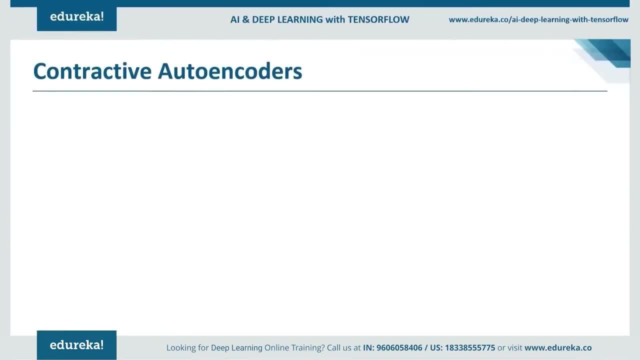 For example, one document could be the question and others could be the answers. now a match The software would make using vector space measurements. The next type of Auto encoders is the contractive Auto encoders. One would expect that for very similar inputs. 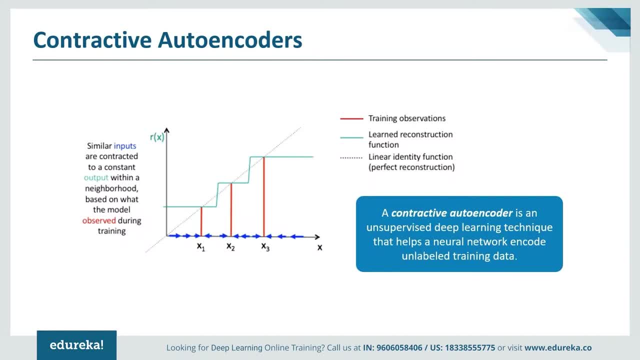 The learned encoding would also be very similar. We can explicitly train our model in order for this to be the case by requiring that the derivative of the hidden layer activations are small with respect to the input. in other words, for small changes to the input, We should still maintain a very similar encoded state. 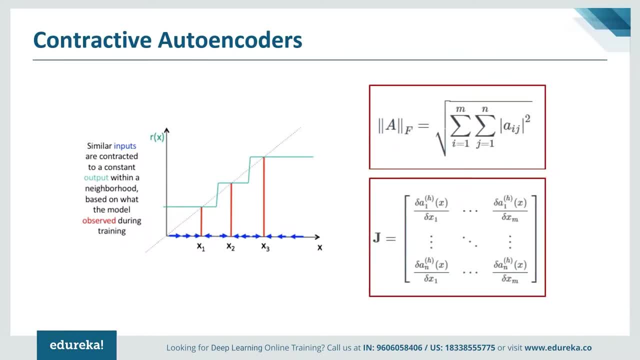 Now this is quite similar to a denoising Auto encoder, in the sense that these small perturbations to the input are essentially Considered noise and that we would like our model to be robust against noise. Now we can accomplish this by constructing a loss term. 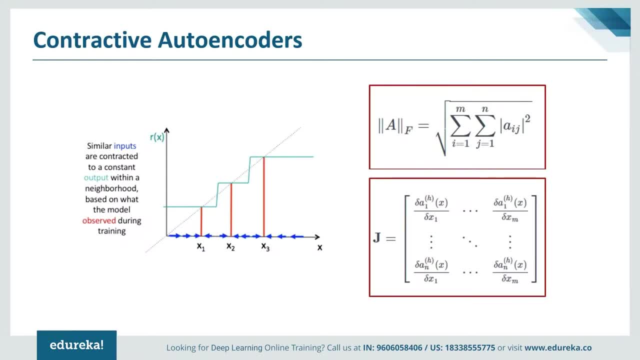 which penalizes large derivatives of our hidden layer activations with respect to the input, training examples, essentially penalizing instances where a small change in the input leads to a large change in the encoding space. now, in fancier mathematical terms, We can craft our regularization loss term. 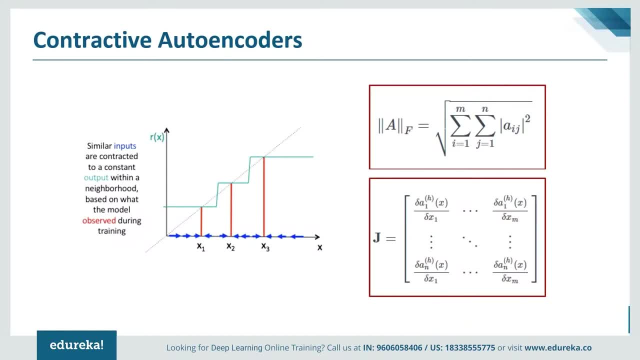 as the squared Frobenius norm of the Jacobian mattress. This J for the hidden layer activations. with respect to the input observations, a Frobenius norm is essentially an L2 norm for a matrix and the Jacobian matrix simply represents all first-order partial derivatives of a vector valued function. now, 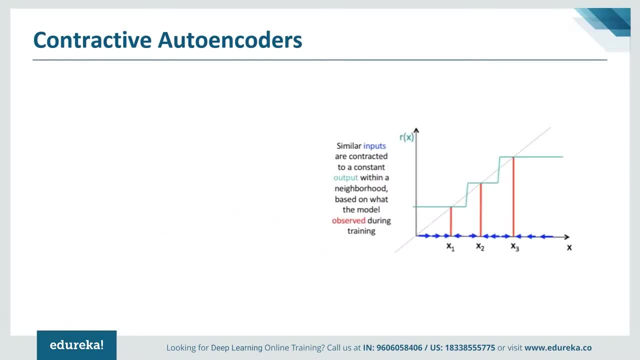 for M- observations and n- hidden layer notes, We can calculate the values using the following equations: So now that we know the various types of Auto encoders, let's have a look at how it actually works. So let's see the code that provides us. 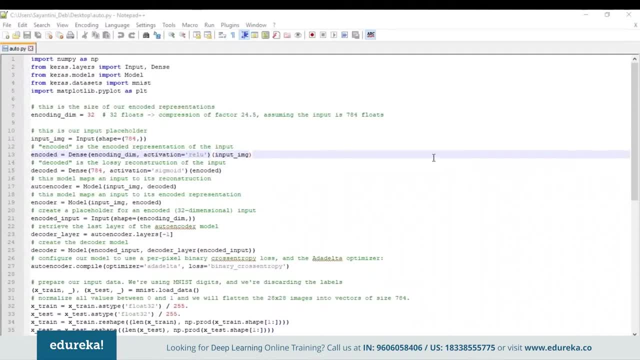 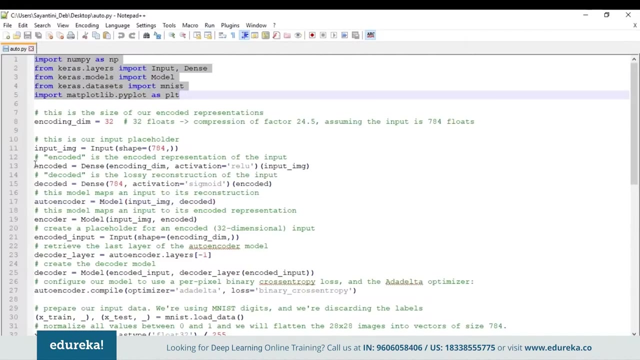 with a reconstructed image. So this is the code for Auto encoder that generates a similar output as the input with reduced dimensions. the packages that are needed to be pre-installed are numpy, Keras and matplotlib. So first we define the size of our encoded representations. 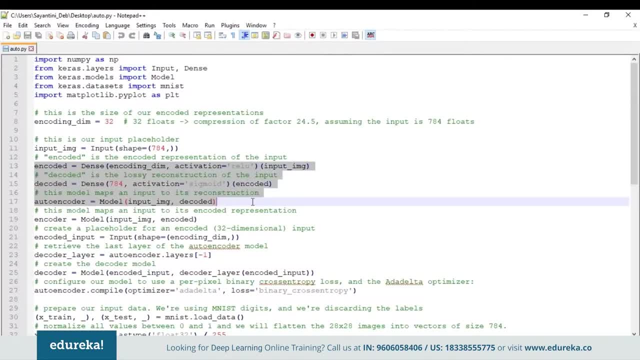 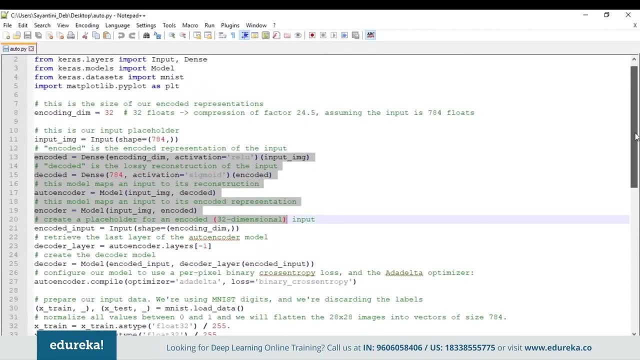 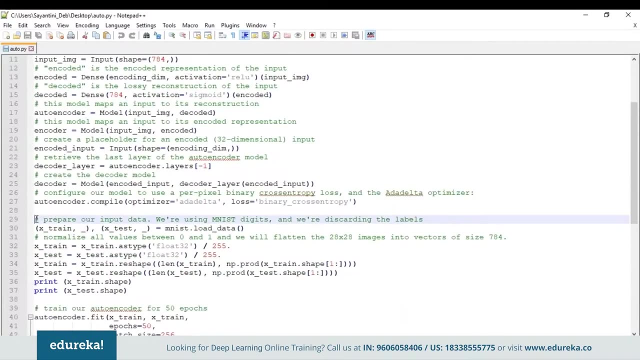 the encoded representation of the input is declared as encoded, while the lossy reconstruction of the input is declared as decoded. The input is then mapped to its encoded representation in order to create the decoder model. next, We have to prepare our input data and normalize all the values between 0 and 1, the 28. 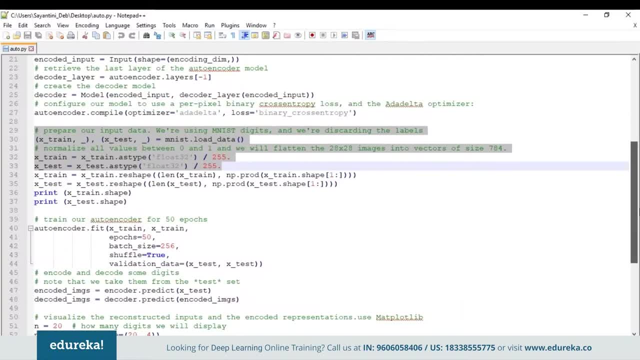 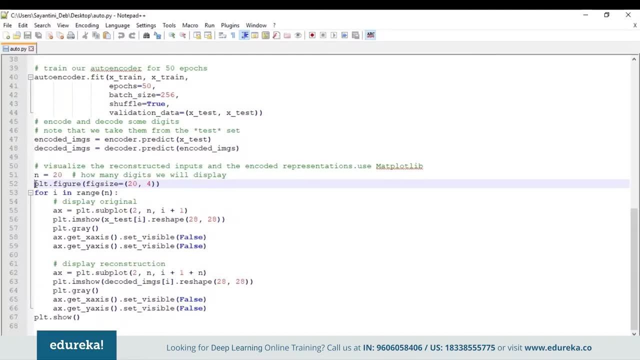 by 28 images will be then flatted into vectors of size 784.. Now, once the data is trained and tested- the auto encoder is trained- It will take certain values from the test set, encode and decode them. now for the visualization of the reconstructed input. 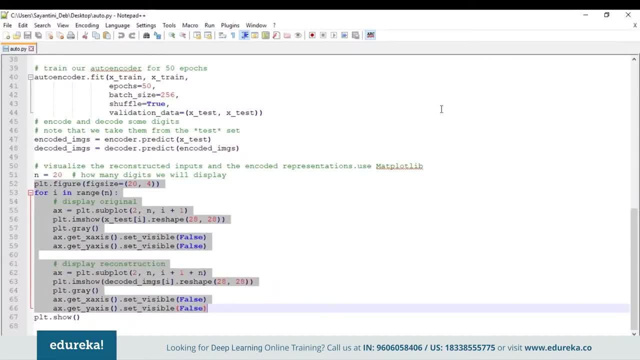 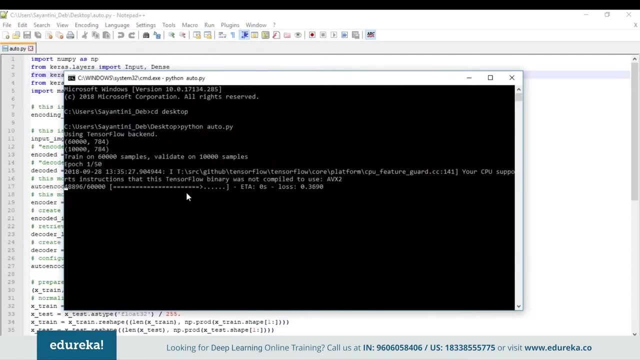 And the encoded representations. it is done with the help of matplotlib library, So let's see what happens when we execute this code. So now we can see that the data is being trained and tested, and this will take a few minutes to complete. Now, once we are done with the training of the data, 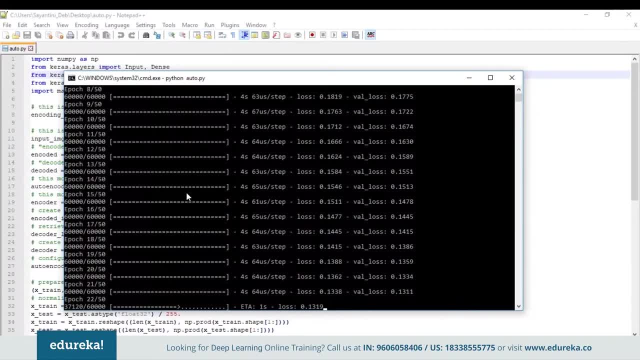 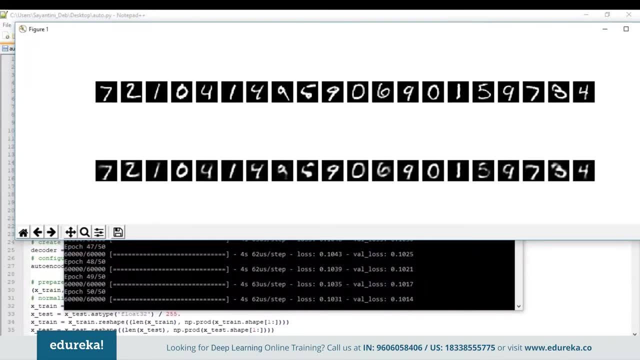 we will have an original image and a reconstructed image as our output. Our output will look like this. So the first row shows the original input image and the second row shows the reconstructed image with reduced dimensions. So now we have seen how an auto encoder actually works. 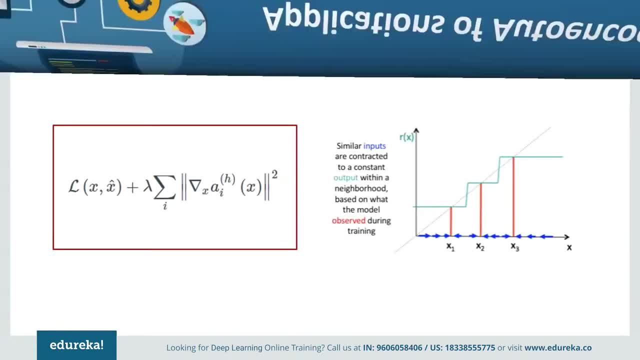 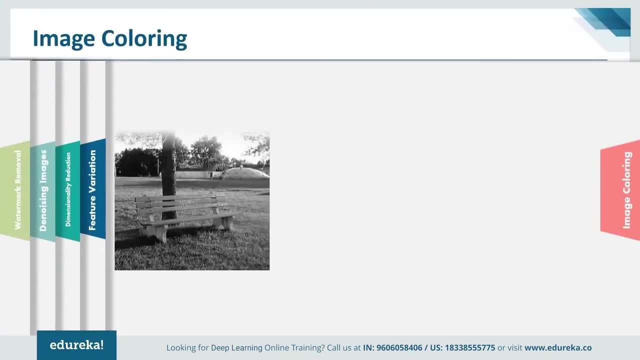 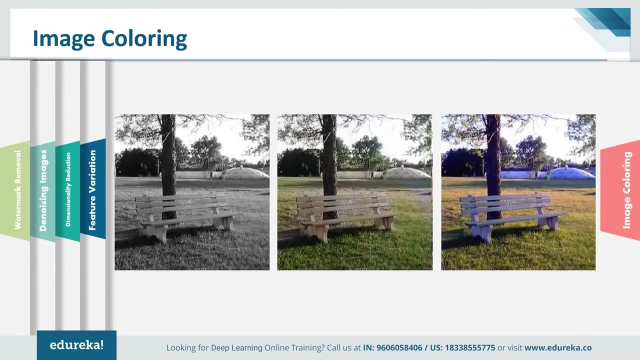 and how it provides us a reconstructed image. So now let's move on to some of the applications of auto encoders. Now, auto encoders are used for converting any black and white picture into a colored image. depending on what is in the picture, It is possible to tell what the color should be. 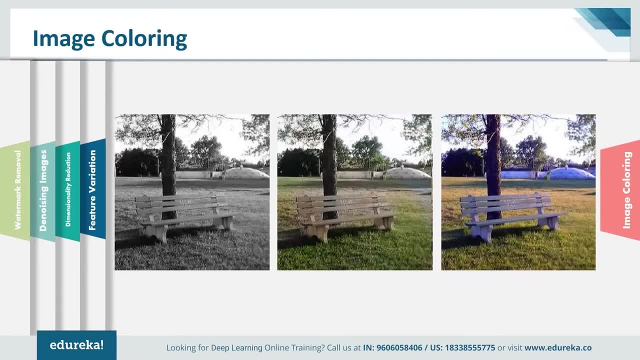 For example, the leaves of trees are generally green, The sky is blue and the clouds are white, So all that is needed to be done is to make a computer be able to do this, and that is where auto encoders step in. The next application is the feature variation. 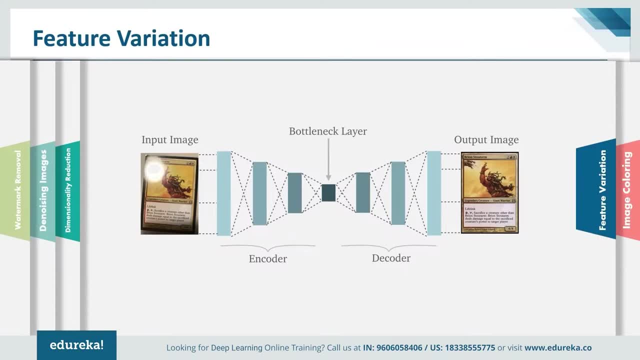 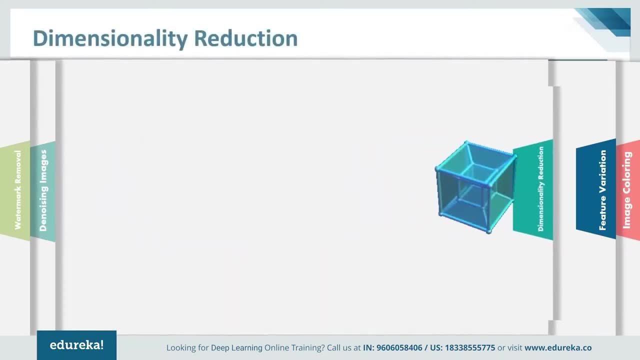 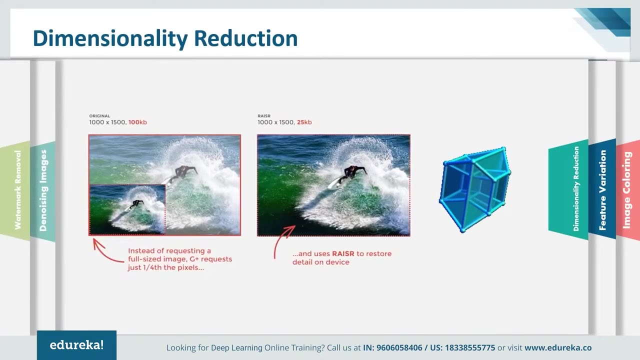 It basically extracts only the required features of an image and generates the output by removing any noise or unnecessary interruption. now, using auto encoders, We receive the same image as the input, but with reduced dimensions. It helps in providing the similar image, along with the reduced pixel value. now, during the training, 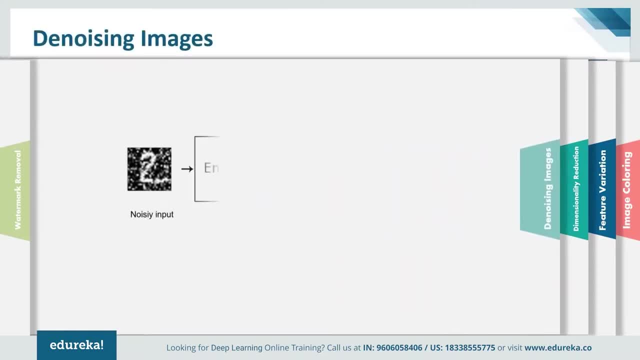 the auto encoder learns to extract important features from input images and ignores the image noises, because the labels have no noises. the input seen by the auto encoder is not the raw input, but a stochastically corrupted version. now auto encoders are also used for removing watermarks from images. 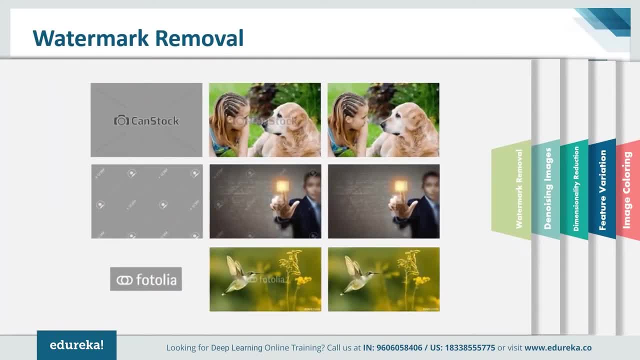 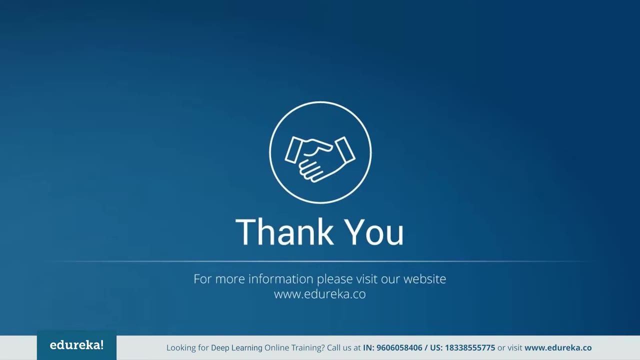 or to remove any object while filming a video or a movie. So now we have reached the end of today's session and I hope you have a clear idea about what are auto encoders and how do they actually work. do let us know if you have any questions in the comment section below. till then, 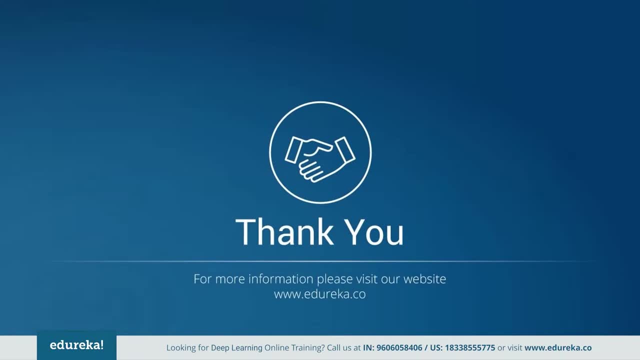 Thank you and happy learning. Thank you.